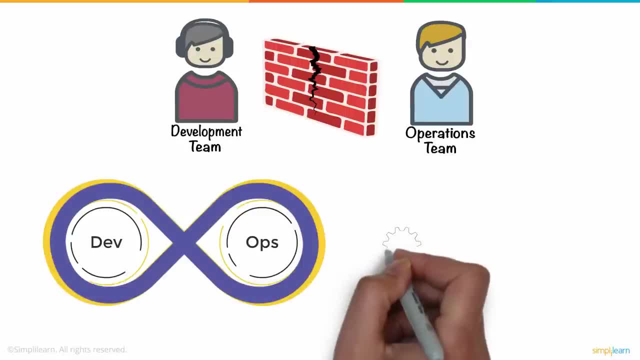 The DevOps symbol resembles an interaction between the two departments, And this is called the DevOps approach. The DevOps symbol resembles an interaction between the two departments, And this is called the DevOps approach. The DevOps symbol represents an infinity sign, suggesting that it is a continuous process. 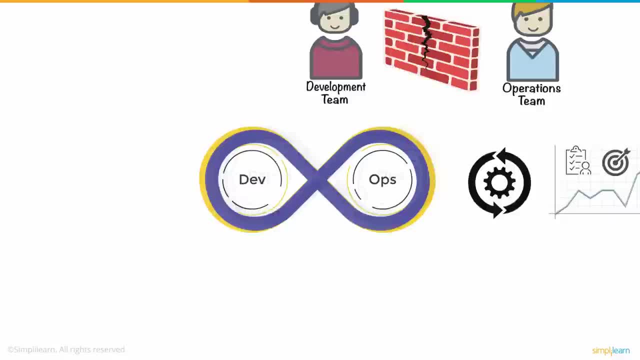 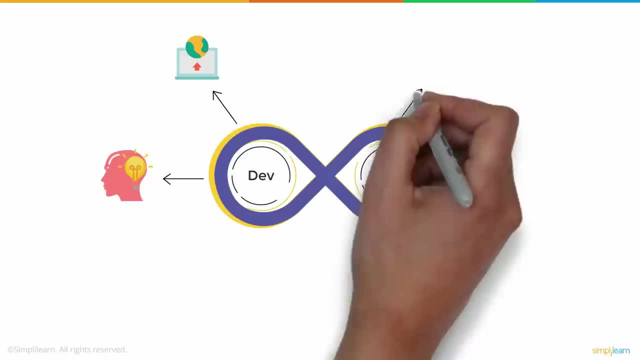 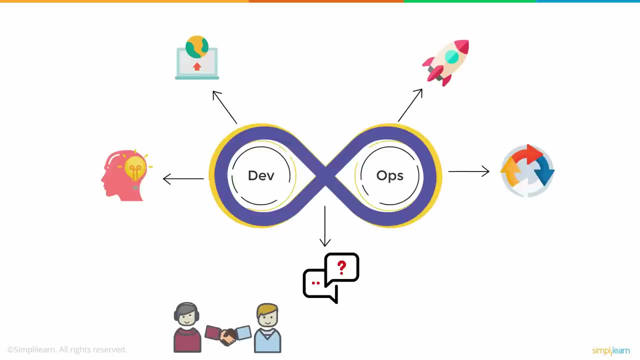 of improving efficiency and constant activity. The DevOps approach makes companies adapt faster to updates and development changes. The teams can now deliver quickly and the deployments are more consistent and smooth. Though there may be communication challenges, DevOps manages a streamlined flow between the teams and makes the software development process successful. 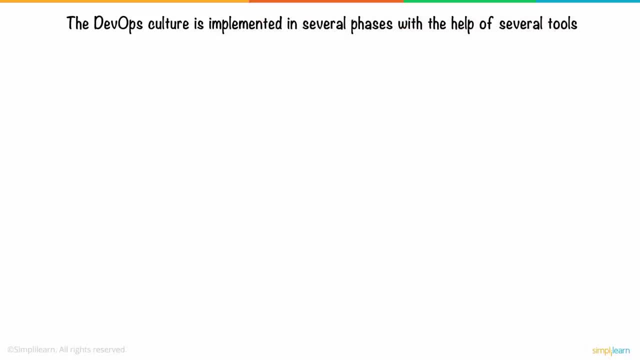 The DevOps culture is implemented in several phases with the help of several tools. Let's have a look at these phases. The first phase is the planning phase, where the development team puts down a plan keeping in mind the application objectives that are to be delivered to the customer. 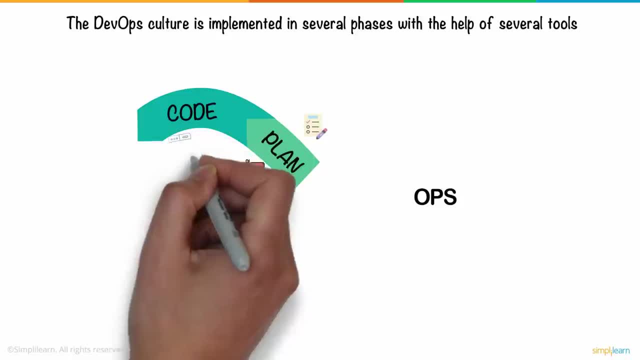 Once the plan is made, the coding begins. The development team works on the same code and different versions of the code are stored into a repository with the help of tools like Git and merged when required. This process is called version control. The code is then made executable with tools like Maven and Gradle in the build stage. 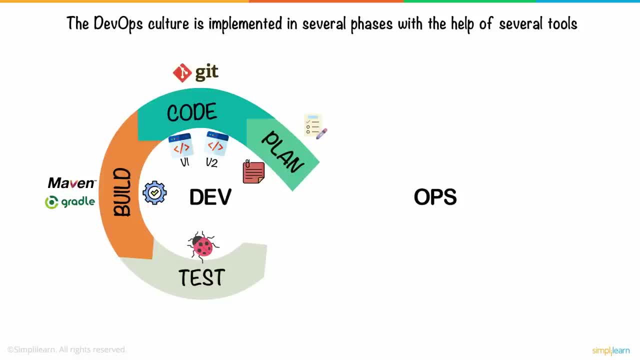 After the code is successfully built, it is then tested for any bugs or errors. The most popular tool for automation testing is Selenium. Once the code has passed several manual and automated tests, we can say that it is ready for deployment and is sent to the operations team. 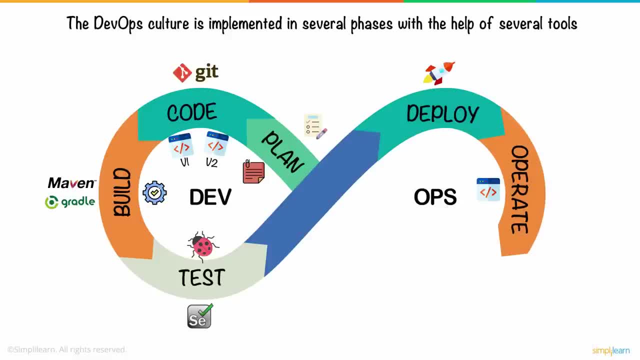 The operations team now deploys the code to the working environment. The most prominent tools used to automate these phases are Ansible, Docker and Kubernetes. After the deployment, the product is continuously deployed to the operating system. The code is then sent to the. 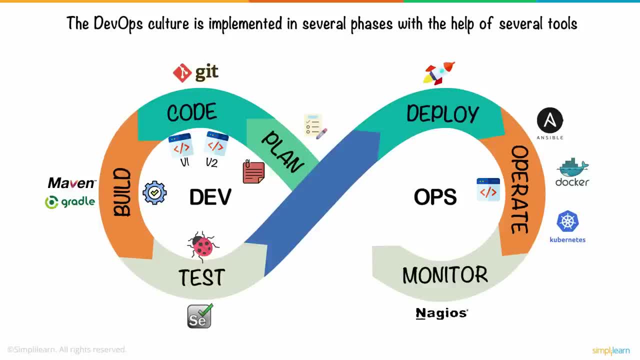 operating team and is then delivered to the operating system. The code is then sent to the operating and Nagios is one of the top tools used to automate this phase. The feedback received after this phase is sent back to the planning phase, and this is what forms the core of the DevOps lifecycle, that is, the integration phase. 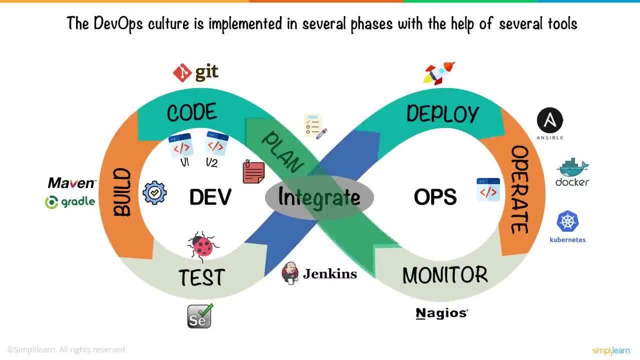 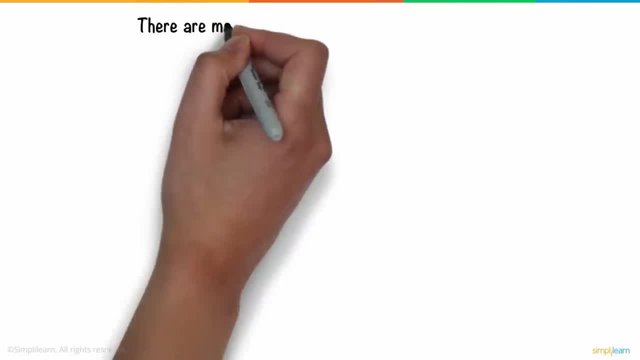 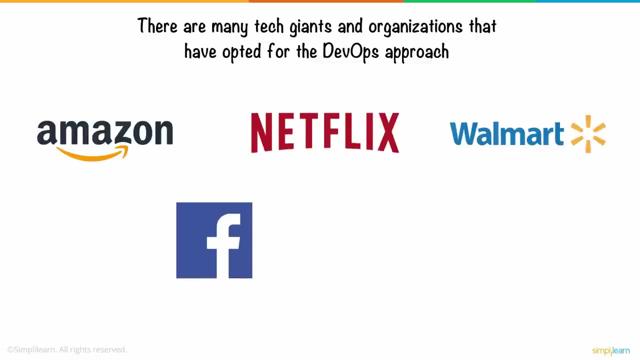 Jenkins is the tool that sends the code for building and testing. If the code passes the test, it is sent for deployment, and this is referred to as continuous integration. There are many tech giants and organizations that have opted for the DevOps approach, For example, Amazon, Netflix, Walmart, Facebook and Adobe.